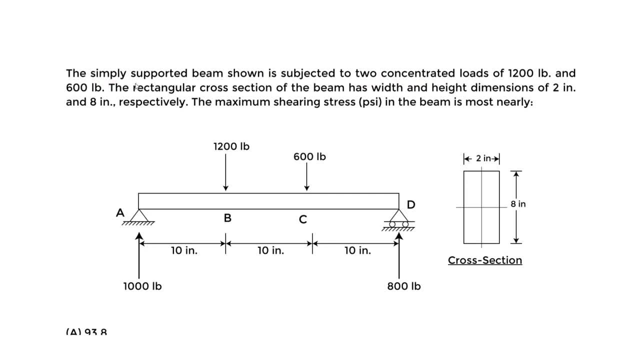 the simply supported beam shown is subjected to two concentrated loads of 1200 pounds and 600 pounds. The rectangular cross section of the beam has a width and height dimensions of 2 inches and 8 inches respectively. The maximum shear stress in PSI in the beam is 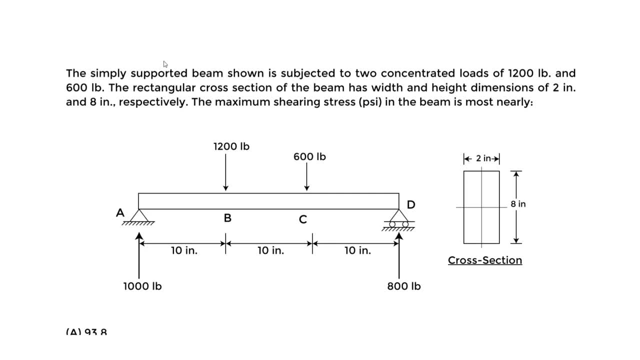 most nearly what. So what we're given is a simply supported beam. Simply supported meaning it has a pin on one end and a roller on the other end- subjected to two concentrated loads of 1200 and 600,. 1200 and 600, these are the external loads, point loads, and we have a 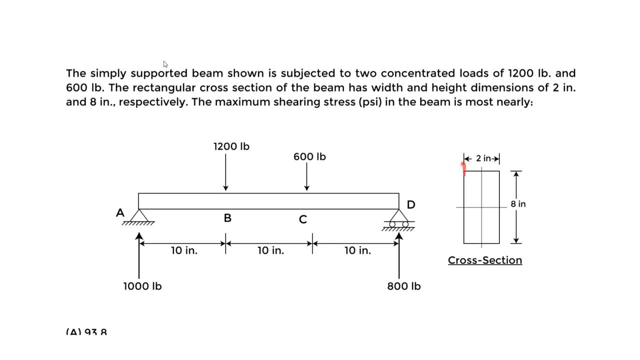 rectangular cross section for the beam right And it has essentially that width dimension which is like the base. So what we have here is a piece of a rectangle- it's 2 inches if you look at it from this view, and the height here is going to be 8 inches for the cross section of the beam. 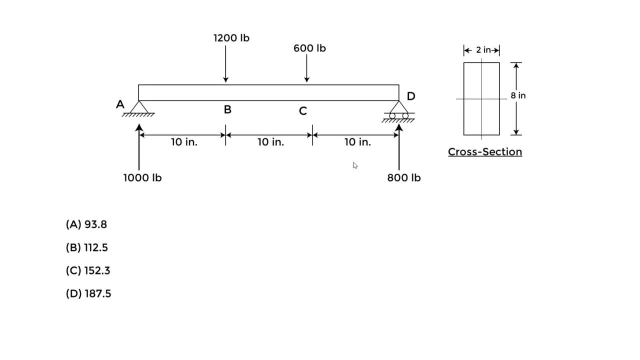 So we want to find the maximum shear stress right in the beam, the maximum shear stress. So let's write that as what we want to find, Find. we'll call it tau max, because we know we use tau for shear stress. right, We use this symbol for shear stress and we want. 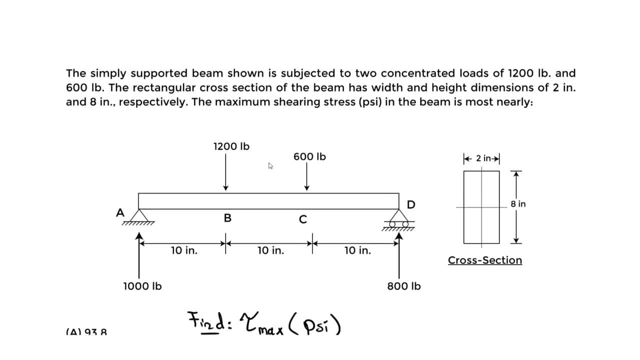 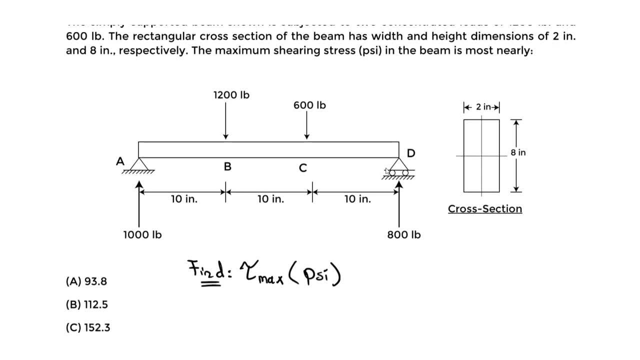 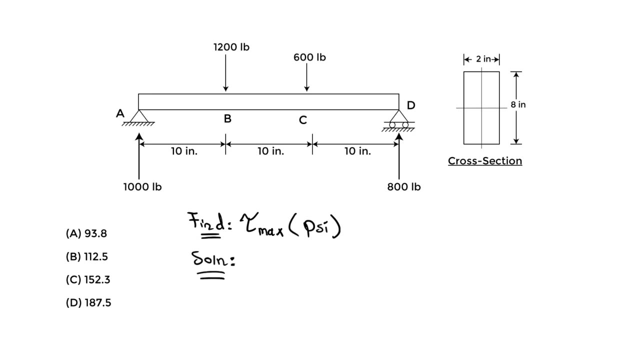 it in PSI, PSI pound per square Square inches. So we're given actually everything in the problem statement, right, We're given the dimensions, we're given the loading. so let's just quickly dive into that solution And what do you suggest we do? So how would you actually solve for that tau, that tau? 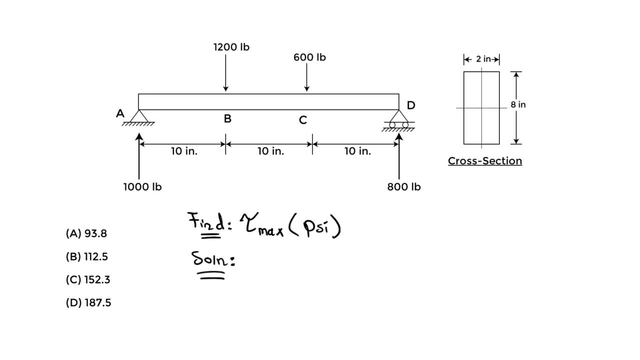 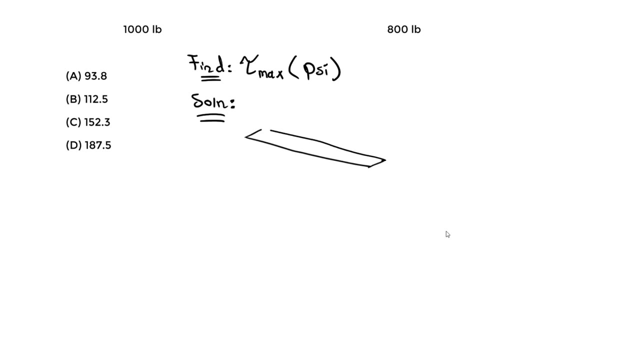 max, the maximum shear stress, basically transverse shear stress in the beam. And I want to say, when they say transverse, all we're talking about here is you have the beam, So let's, let me actually draw that. You have like a beam here and for this beam you would 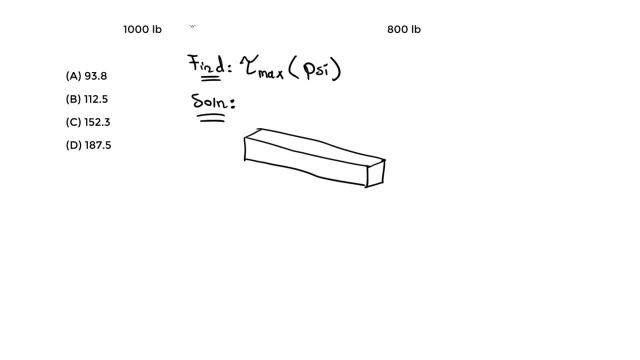 have like a shear stress and that transverse direction, meaning it's going to be in this direction. So we find that shear stress right. This is the shear stress that we're going to solve, for, Most importantly, we're going to find the tau max right, The maximum Tau. 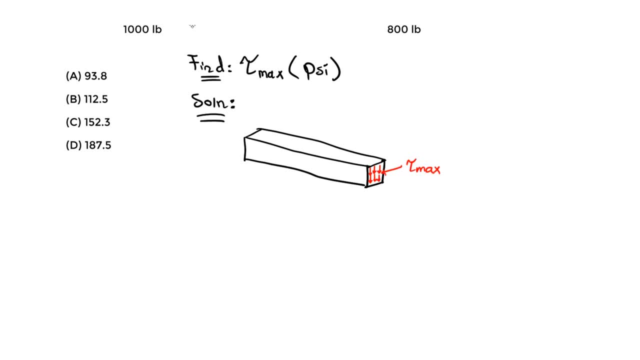 max. So what we can do is actually just use the FE handbook equation right, The transverse shear stress equation, and it's going to be under what section? The stresses in beams, Stresses in beams. So it's a whole section. If you do control F or control shift F, it 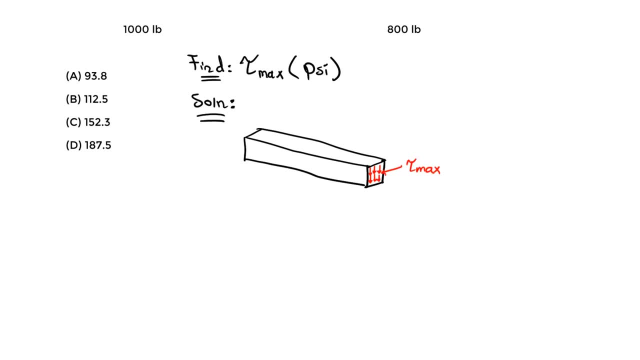 should come up as a section. You type that stresses in beams and it has the normal stress. but that's not what we want, right? We do not want that maximum normal stress or the normal stress at any location. What we want is the shear stress. 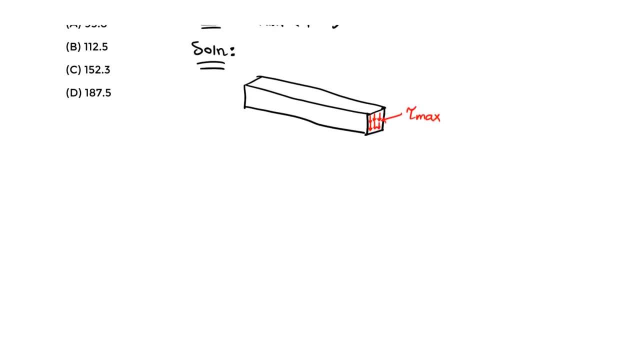 The transverse shear stress. So let's write that equation first. So we're going to say that tau max is going to equal to the V Q divided by IB, IB. So here V is going to be the shear force right. V is the shear force, Q is the first moment of area and 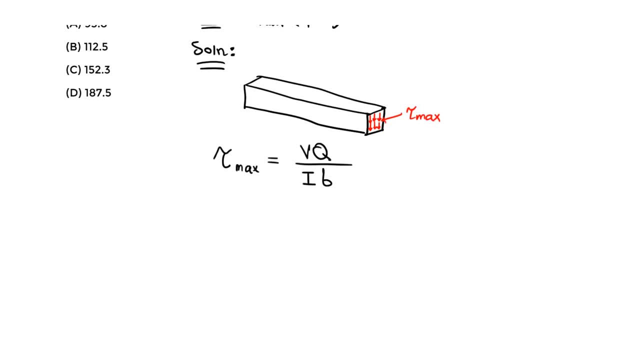 we know I is going to be the moment of inertia. Then B is going to be just simply the width of the cross section. So B in this case is quite simple. It's just two inches, right. But we know here that let's work one by one. So let's take it one by one. Let's look at: 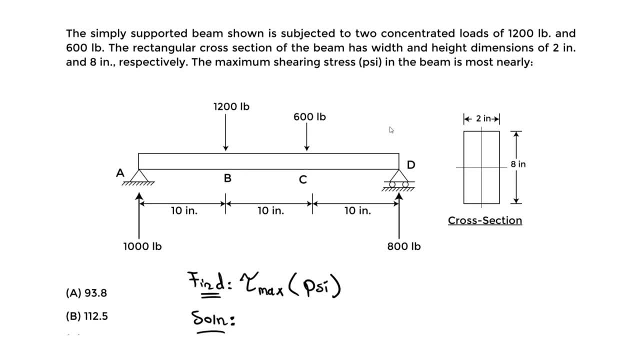 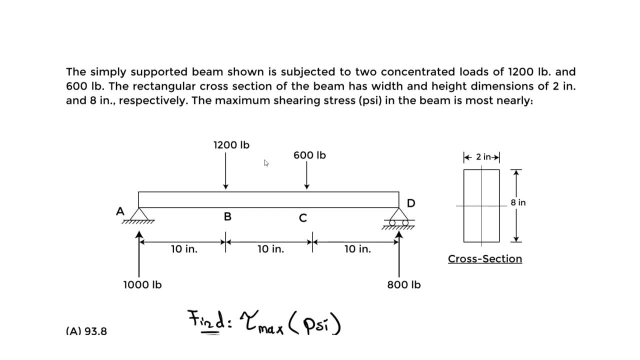 V. So V is the shear force. Here we're not really given an exact value, right? We're not given that shear force. So we do not know. We do not know that shear force. But one big hint is they're telling us: you want to find the maximum shear stress. That tells me okay. 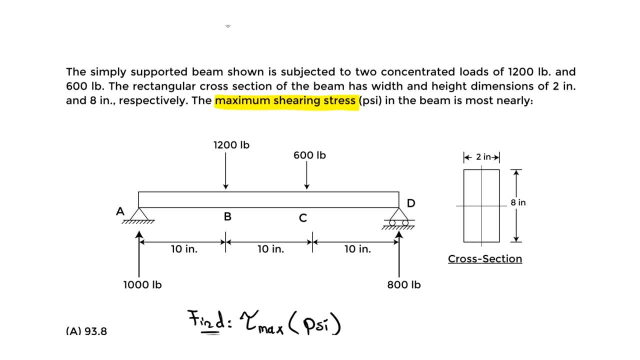 V occurs when, When we have that maximum shear force, that maximum vertical shear force, And how would we get that shear force From the shear diagram? right, You have that shear moment diagram, but all we're going to do here is look just strictly at the shear diagram. 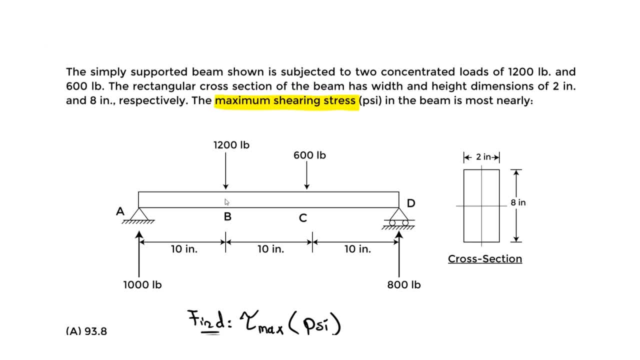 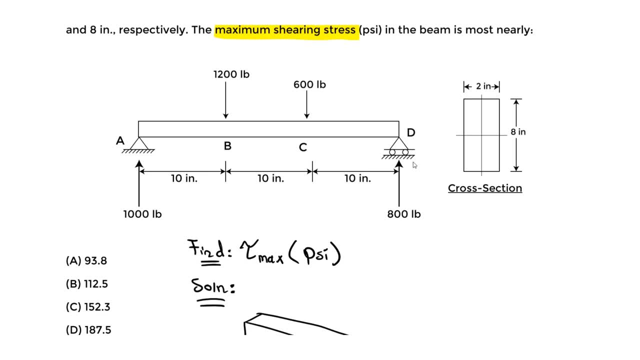 and get the maximum value for the shear force drawing that shear diagram. So if we draw the shear diagram real quick, in this case, we're given all the loads, right, You're given the reactions, So you can do that real quick, right, We can do that, And what we can do is just draw the 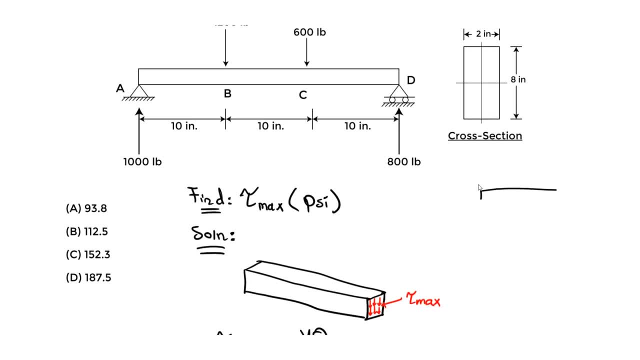 beam here And we know we have the reaction here is 800. And the reaction here is 1,000. Those are given for like a FE type question. This is 1,200. And this is going to be 600.. 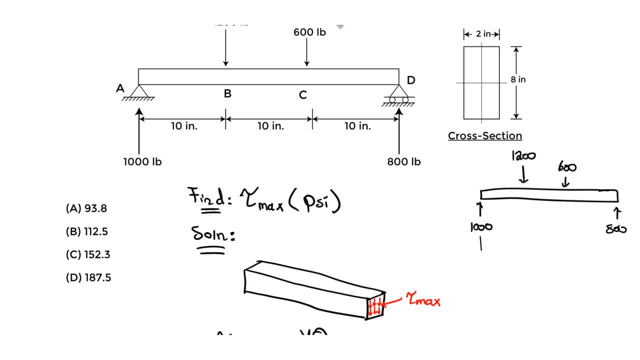 So you just draw that shear diagram. So if I draw that shear diagram, you can see that here zero is going to be this axis And we know that zero is this And we're drawing the shear force. Let's call it V And the units will be what? in this case pounds. 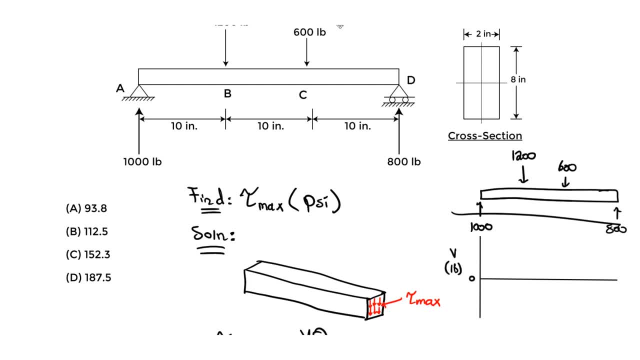 right Units of pounds. So at this end you start from left to right. So we start here And we know at this where we have A that pin. it tells us: go up The arrow points up. So we just go up how much. 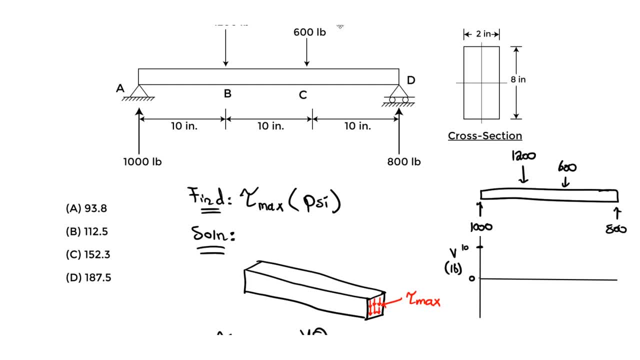 1,000,, right, 1,000 pounds, We go up 1,000.. Starting here, we go up 1000, then we move across. we notice nothing is happening. right, Picture you moving there, nothing is happening. 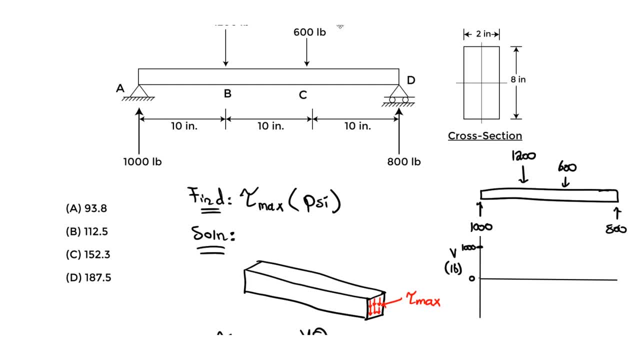 So you just stay flat. So it's just going to be constant. So it's constant all throughout. constant, constant, constant, constant until we hit this 1200, which is essentially here at B, And at that 1200, it tells us, go down 1200. 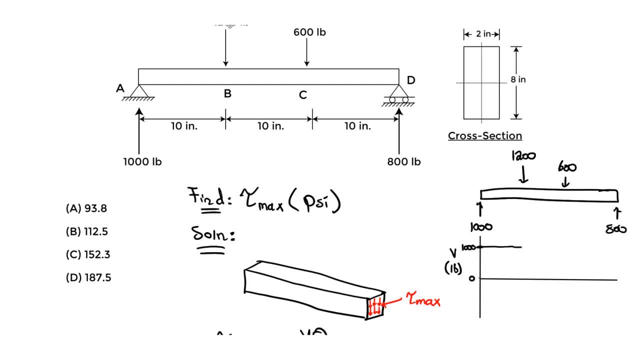 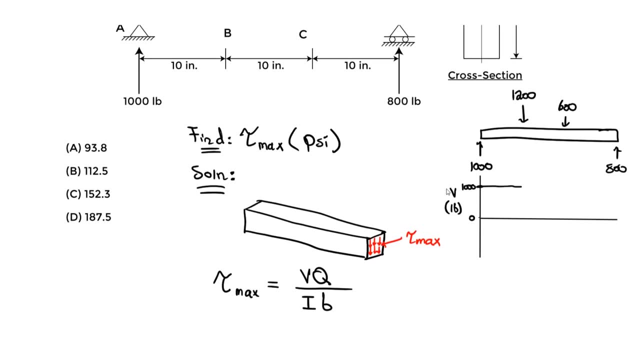 from where The 1000, right From the point we're at, which is 1000, go down 1200, and that brings us to what It's going to bring us: to negative 200.. So that brings us down to negative 200. 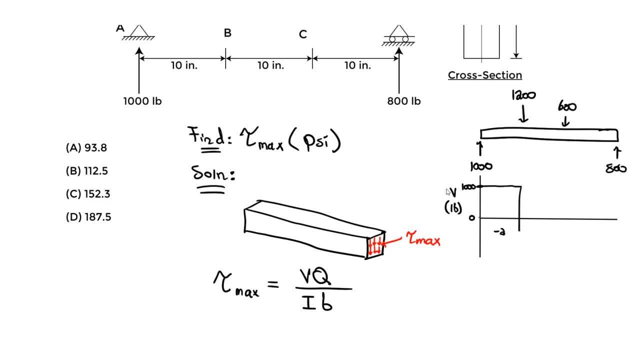 So it's just a vertical line to negative 200 pounds. So now we are essentially here, right, And then we keep moving, keep moving. nothing is happening. So we just stay flat, flat, flat flat. But here we notice we hit that 600.. 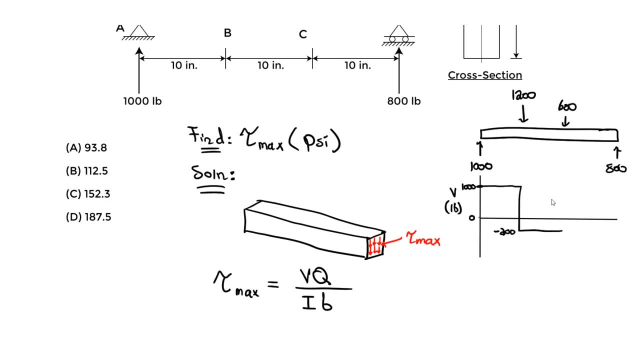 That tells us: go down 600.. Somewhere the negative 200. So you take negative 200 minus 600, and that gives us how much Negative 800. So that's just vertical negative 800. Then now you move across, cross, cross and we end here, right. 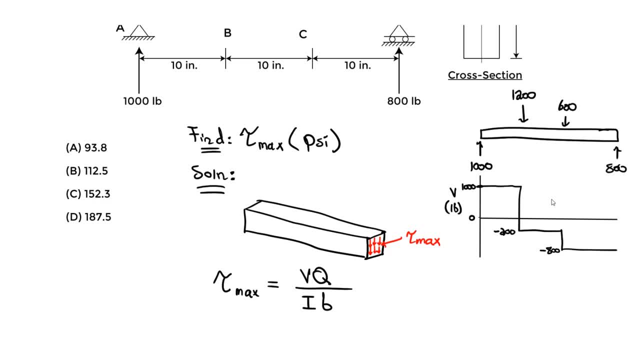 So flat, flat, flat, flat. And then this tells us, it points up, So it tells us: go up positive from the negative 800. So we're at negative 800 here, We add 800. And we end at 0.. 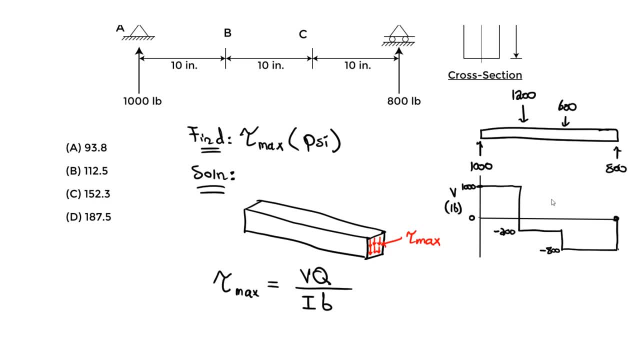 That tells us we did this thing right when we end back at 0, right. So now this is the shear diagram And all we do, just like what we stated. you just take the max value, So this is actually the V value. 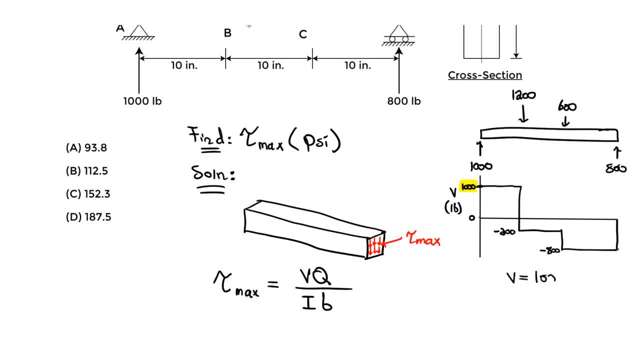 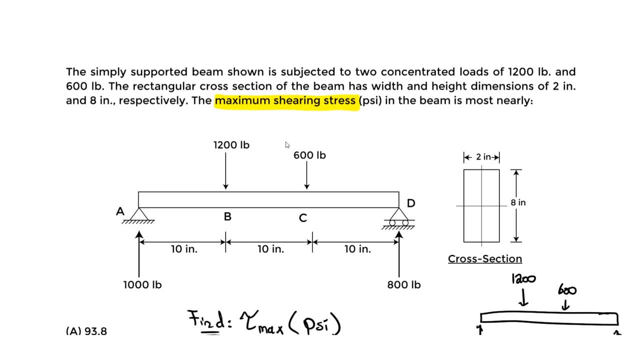 This is going to be the V value we use. It's the maximum value of 1,000 pounds Because we want to find once again. the problem statement says maximum shear and stress, So use your maximum shear and force. So that's the V value you would have to use, right? 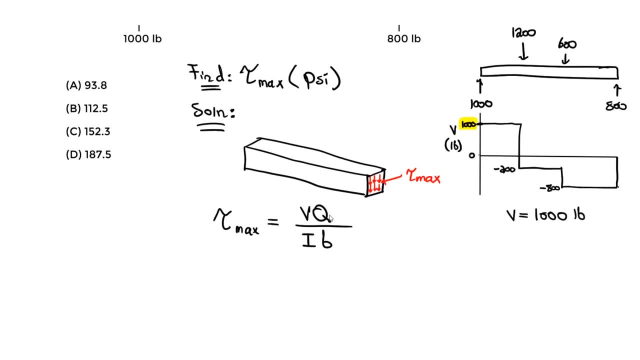 That 1,000.. And that's what we're going to put in there. So we took care of that right. That one's done So. now let's move on to the next one, Q. So Q can be complicated. 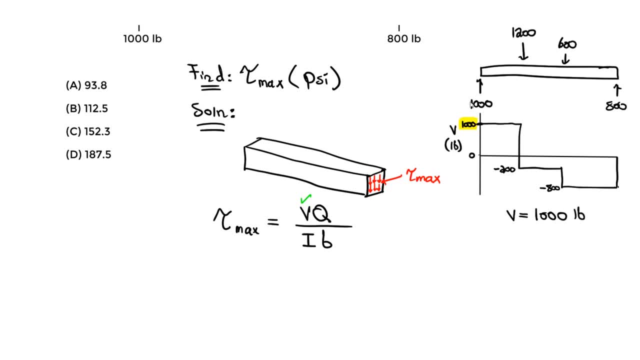 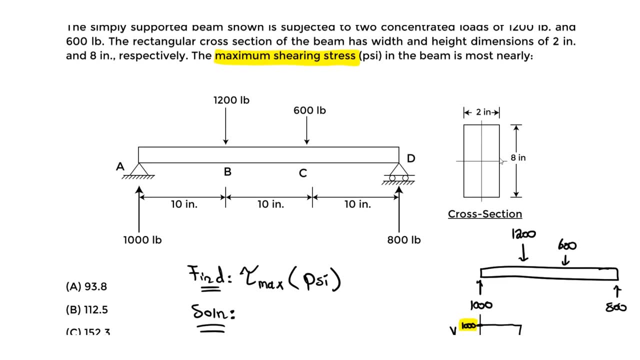 Q can be complicated And we'll learn it for this simple example. But you can apply the same procedure to I-beams, trapezoid shapes, circles or T-beams, non-symmetric I-beams and so on. 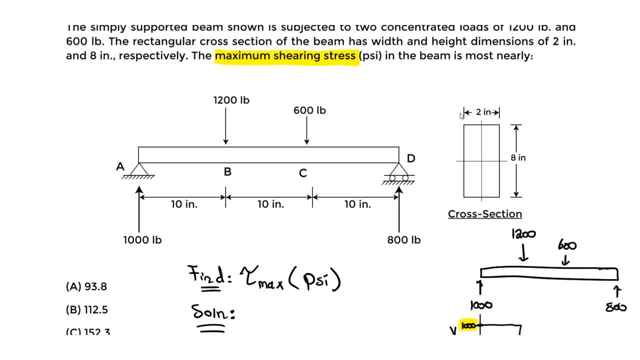 But this one's going to be relatively easy. It's relatively simple, right? Because you just have a rectangle, and it's symmetric, about the middle axis, And that middle axis is also called the neutral axis, the middle axis. So now we know we need to find Q, And in the handbook it says Q is the first moment. 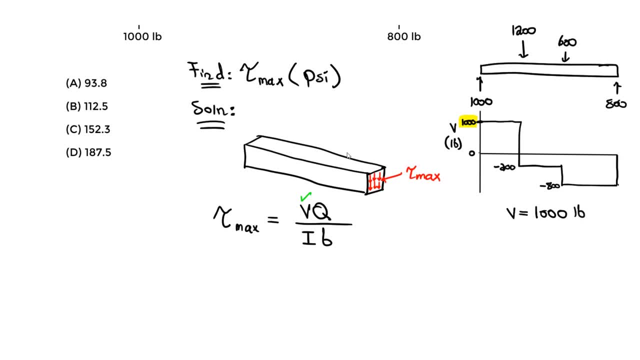 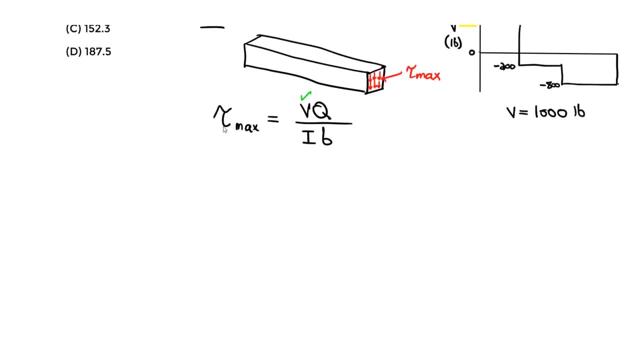 of area above or below the point where the shear stress is to be determined. So that's going to be Q. So let's write the equation. It's the first moment of area. It's going to be A prime OK Times Y, prime bar. 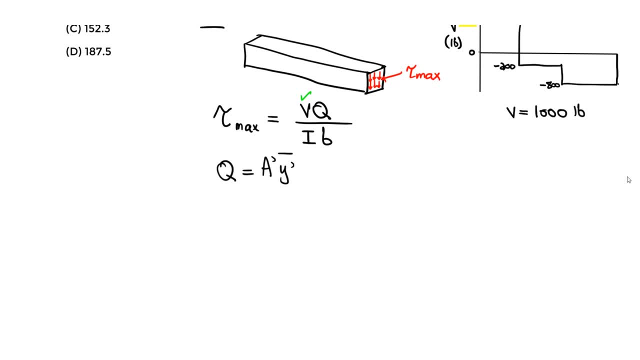 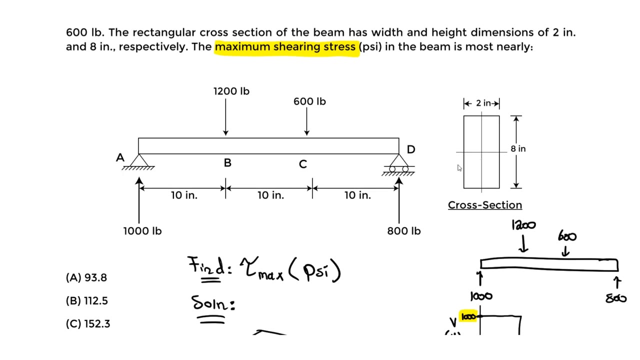 So it says: be careful with the wording. It actually tells you what to do. in that statement. It says first moment of area above or below the point where the shear stress is to be determined. So now you're like: OK, where the shear stress is to be determined. 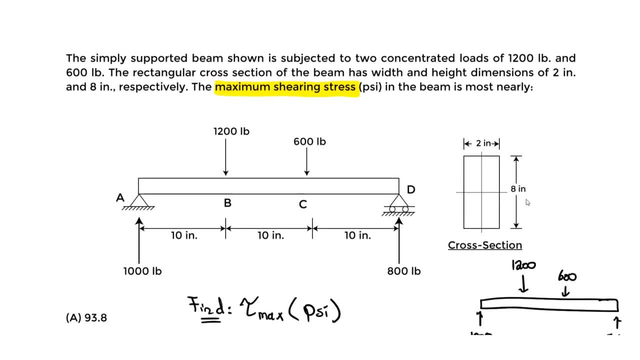 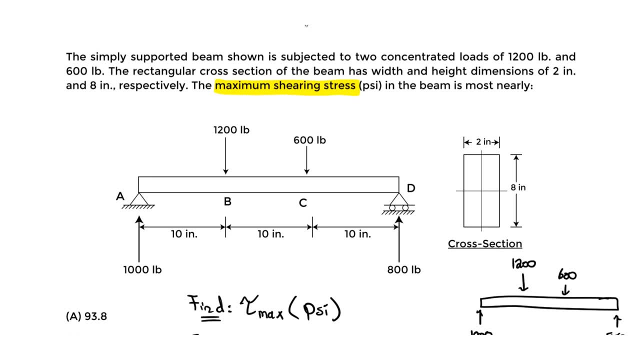 Where is the shear stress to be determined? If you look at the cross-section, let's focus on the cross-section: Where is the shear stress to be determined, Where the maximum shear stress occurs. So now you actually have to think about that stress distribution, the shear stress distribution. 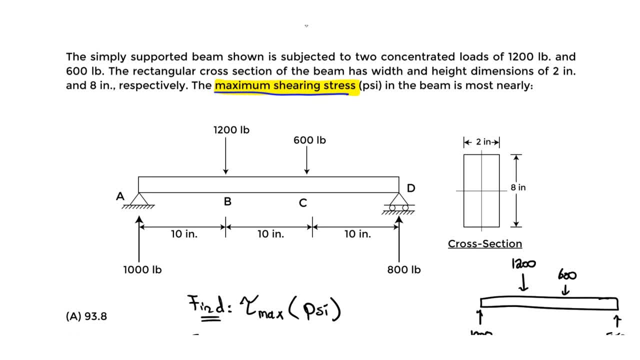 Not the normal stress distribution. That's different. We look at the shear stress distribution And we know the shear stress distribution for a simple shape like this is just going to be parabolic And it's maximum at the neutral axis. And if I draw that, for us it looks something like this: 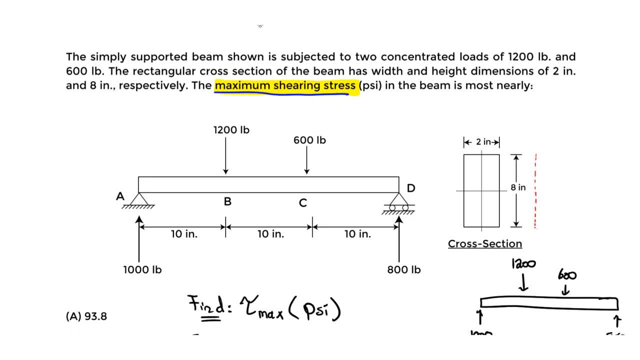 So let's say, we start. this is like where we have zero here, zero here, We draw a parabola. right, You draw that parabola, You draw the parabola which should be. it should be symmetric. 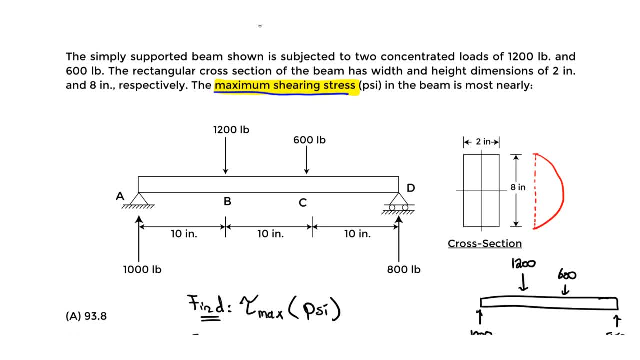 So this thing should be symmetric. about what axis? The neutral axis. So this is the neutral axis, This whole thing is the neutral axis. We'll call it NA neutral axis. And what's interesting is the maximum shear stress occurs at that neutral axis, tau max. 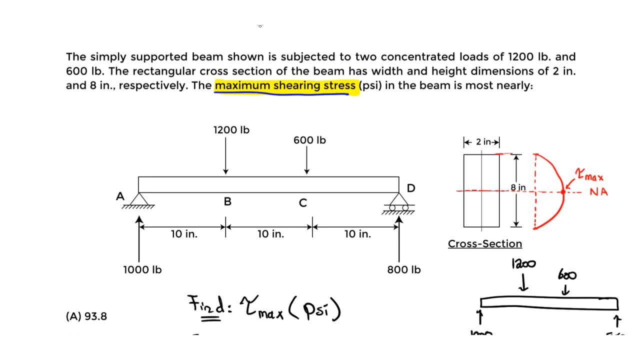 which is what we want to find Here at the top, at this top and at the very bottom, like at the edges, it's zero, Tau is zero And you can like, if you picture the normal stress distribution, you can pause the video. 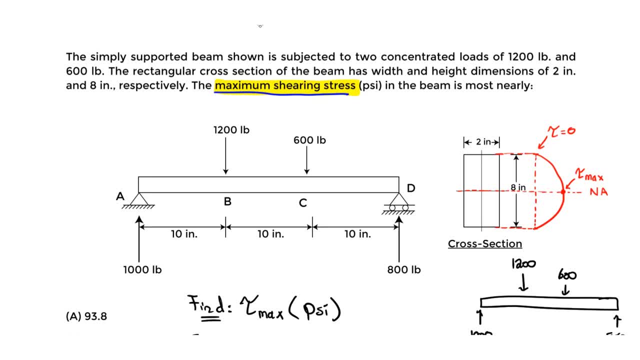 and try to draw that or Google it. It's basically the opposite. right, Because at the top fibers they're normal stress, It's actually maximum, right? The compression. well, if you have, in this case, positive bending, you have the positive. 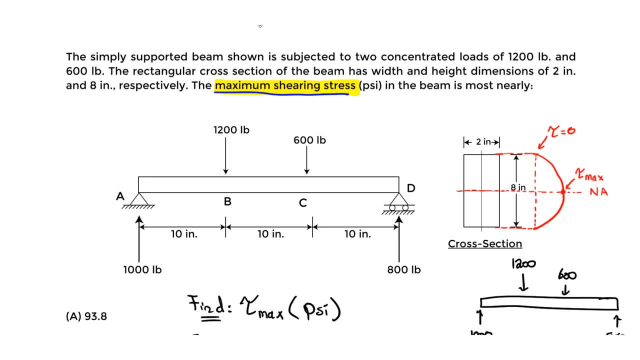 on top, So you have the compression on top and tension on bottom. So it's actually like the opposite, right The opposite, And that one's actually linear right For the normal stress distribution, when we find the moment right, When you find the maximum moment and when you use the normal stress equation. 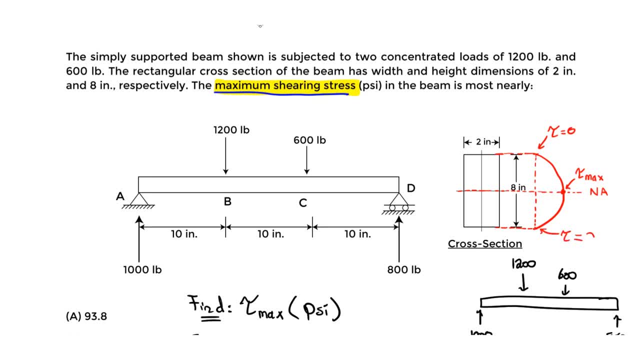 But note that at the bottom and top the tau is zero. Tau is zero And this is your stress distribution. Again, at the neutral axis it's maximum: the shear stress, the transfer, shear stress. So this is what we have. 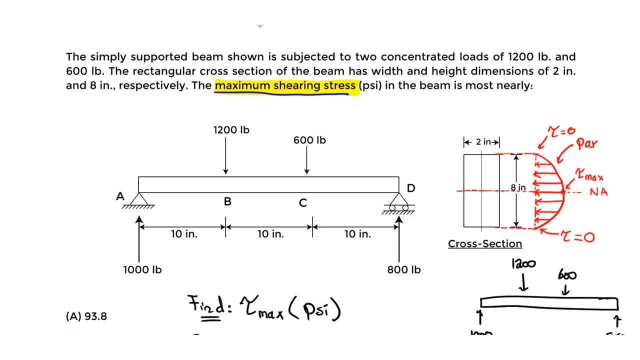 And that's how the stress distribution looks like. And I want to right: We said it's parabolic, right? Parabolic It's a parabolic distribution for the shear stress, for a simple shape like this one, which is going to be a rectangular beam in this case. 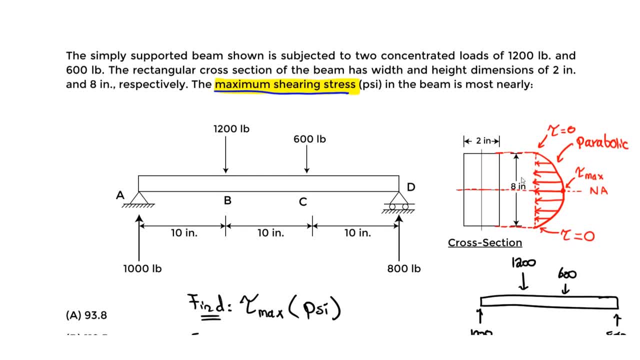 So now that's going to be that, And now We know where that point is right. We know it says, above or below the point where the shear stress is to be determined, The first moment of area. We know where the point is. 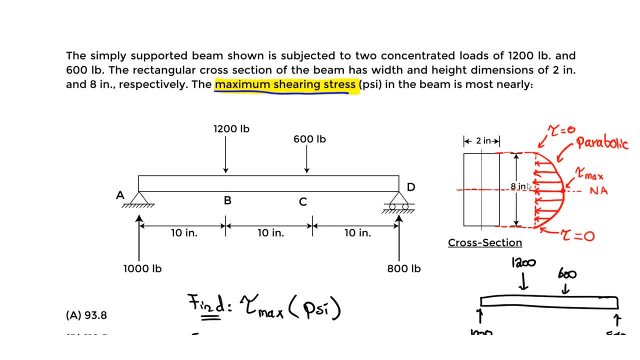 It's going to be there. It's going to be at this point, right, Because that's where the maximum is. So now all you have to do is pick an area above, or pick an area below, And here or there, just the same right. 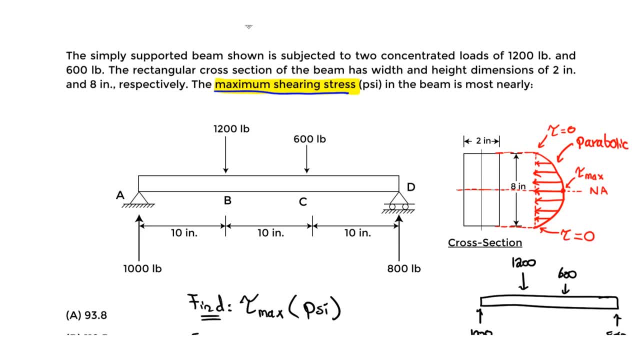 So what we're saying is: we know the maximum shear stress occurs here. That's the point where it is to be determined, right, That's the point where we want to find it. So we pick an area above that, whether it may be this area or you can pick the bottom. 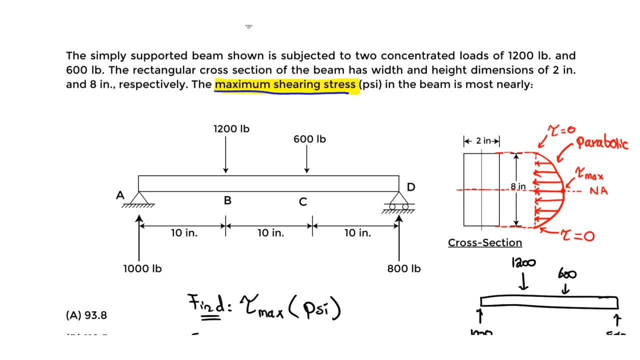 area. They're the same right, They're going to be the same areas, And think of this as like taking the whole area. You start here from zero, You take the whole area until you get to the maximum right, So you take this whole area. 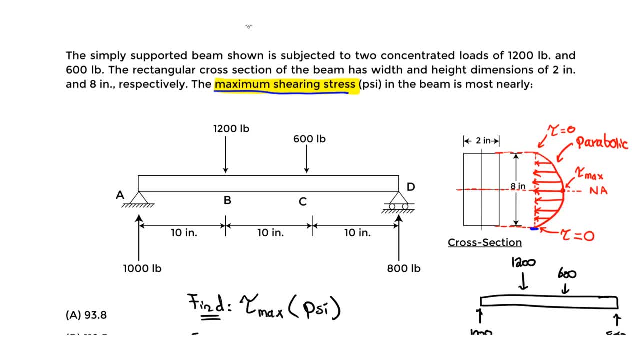 Or you can do the same here. You start at zero, take the whole area until you get the maximum. You can use that area above or below, right, Above or below, where the shear stress is to be determined, which is at the neutral axis. 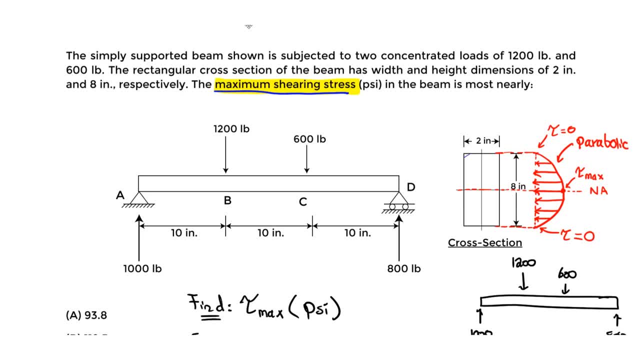 again because we want to find that maximum shear stress. So here I'll just use the one above. It's actually the same in this case, But that's going to be the area that we're going to look at. That's going to be the area. 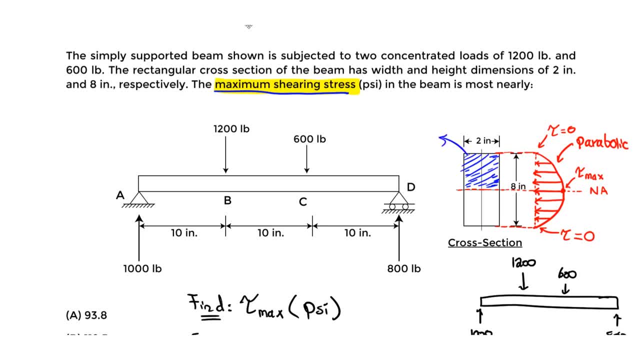 And let's actually find the area. That area is actually the A prime value. That's going to be the A prime And for A prime We just take the area of that shape right. So the area for that shape, we know, this dimension is how much? 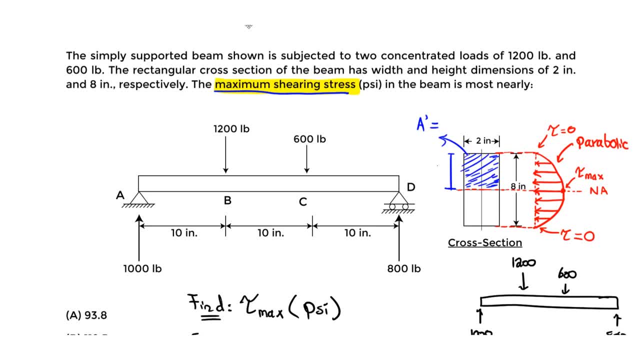 We know the whole thing is 8.. That has to be 8 divided by 2, which is 4 inches. That's 4 inches. So the area of this shape is just 2 times 4, right, 2 inches times 4 inches, which is 8 inches squared. 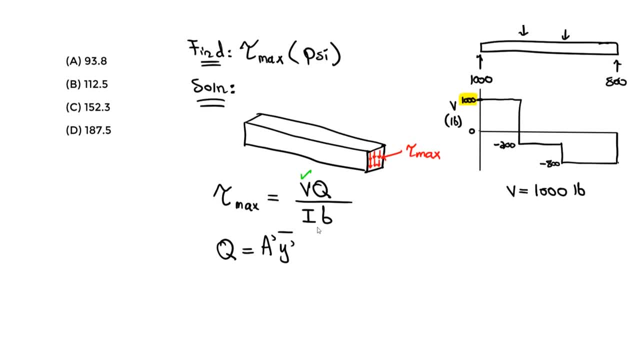 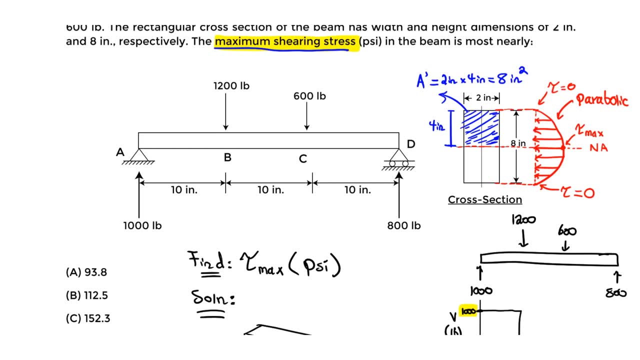 So now we're done with A prime. So we just found A prime right. We found this Now: Y prime bar. Y prime bar, That's actually defined right. It's going to be the distance from the neutral axis to the centroid. 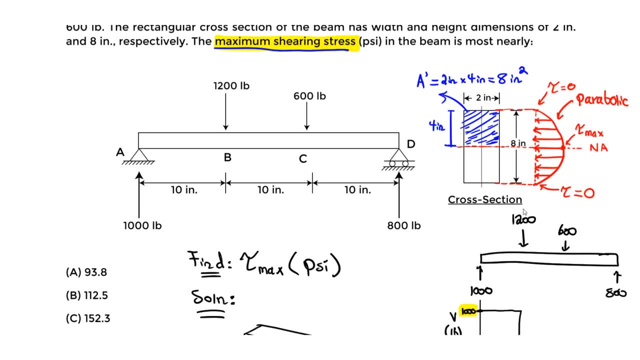 Distance from the neutral axis to the centroid of the area. Of the area we denoted in blue here, right Distance from the neutral axis to the centroid of the area. So now let's actually denote the centroid of the area. Call it here. 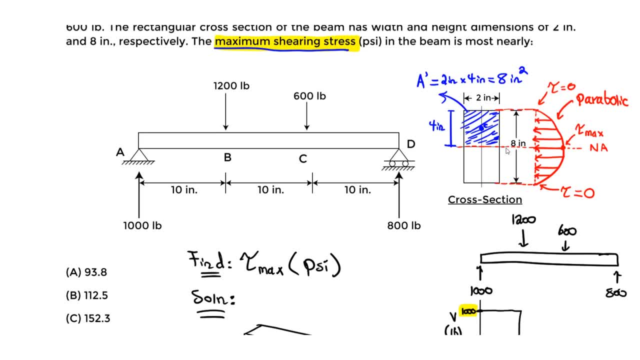 That's going to be the centroid of the area, which is like that center right. It's just 4 divided by 2 from the top And 4 divided by 2 from the neutral axis. So it's going to be this distance actually, right. 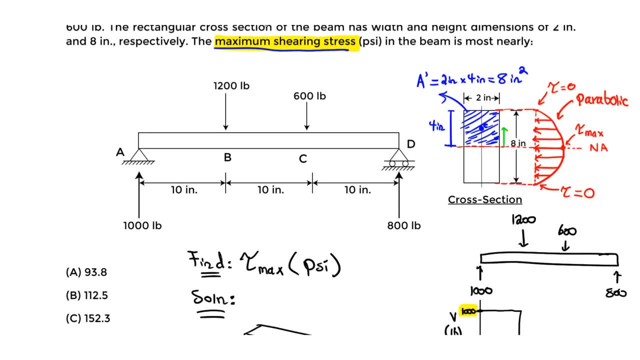 That distance, Y bar prime is going to be this distance. It's going to be that distance to the centroid of the area that we're looking at. So that's going to be Y bar prime, So Y bar prime, And that's going to be how much, if you actually find that. 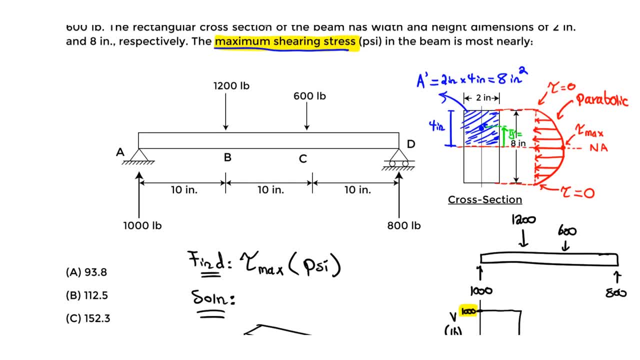 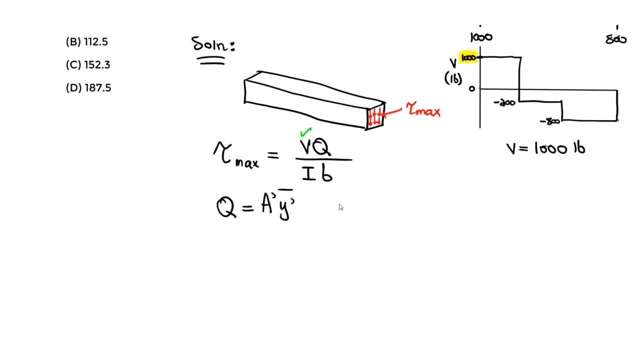 You just take 4 divided by 2, right, Take 4 divided by 2 and you get 2 inches. That's going to be 2 inches. So now we're done. right, That's going to be the first moment of area, because we have A prime. 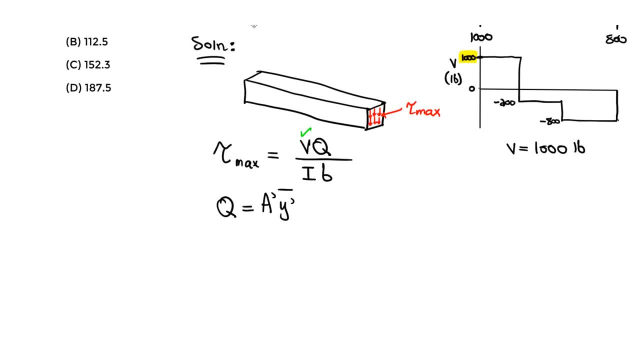 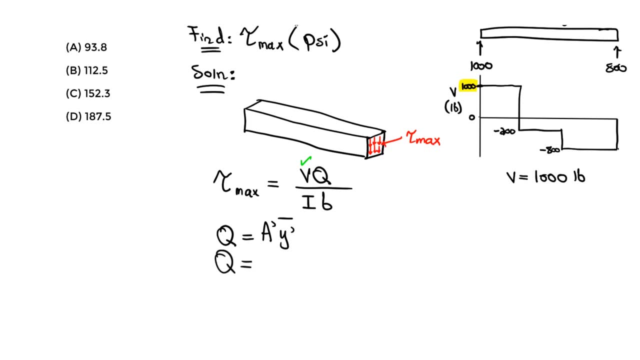 We have Y bar prime, So Q, let's actually solve for that. So A prime is going to be how much A prime? we said it's 8 inches squared And you multiply by the Y bar prime, which we said is just the 2 inches, right? 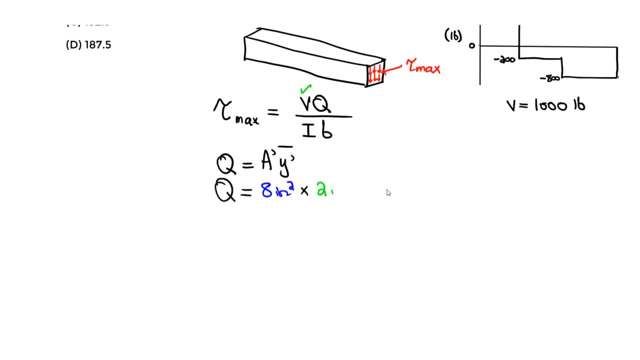 That's going to be the 2 inches. That's going to be the 2 inches there, And notice how inches squared times inch is going to be inch to the third. Those are the units for Q, the first moment of area. So you take 8 times 2 and you get 16 inches to the third. 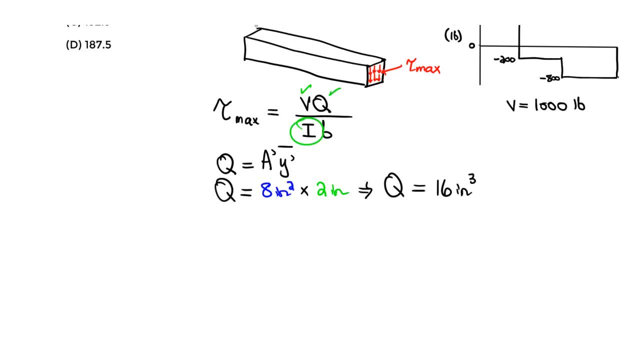 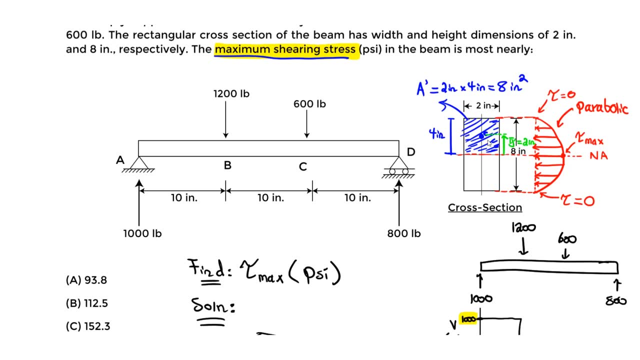 And that's what we will plug in there. So we're done with Q. We're almost done. I, in this case, is what? How would you find I for a rectangle? You just use the statics tables, right, And in this case, you have bending about the X axis. 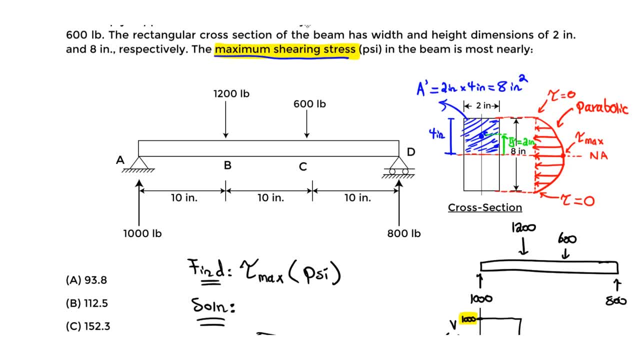 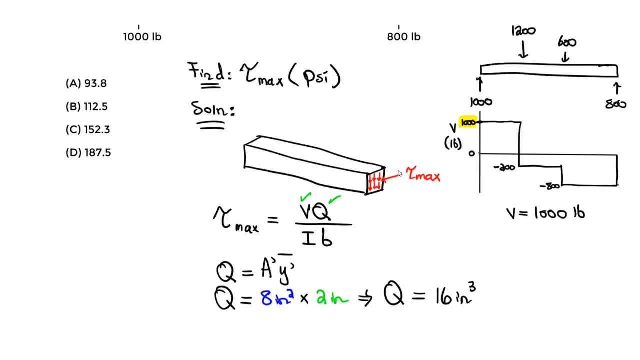 Well, the neutral axis. You have bending about the neutral axis, in this case, the neutral axis being that which is actually like the X axis, which is like the X axis, And you can picture it like in this case, if I redraw this thing, you have like a beam. 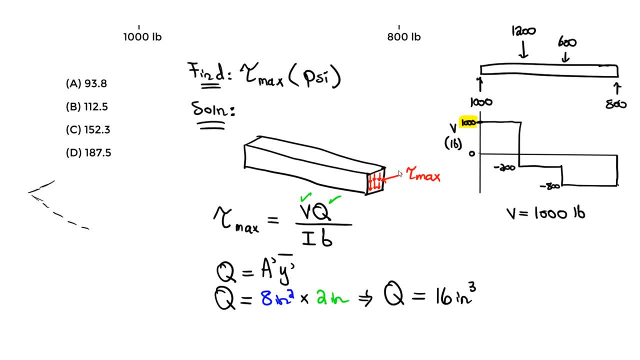 that's trying to bend about like the axis which is like the neutral axis, And it looks something approximately like this right? So it would look something like that And you have bending about that neutral axis which is going to be this way. 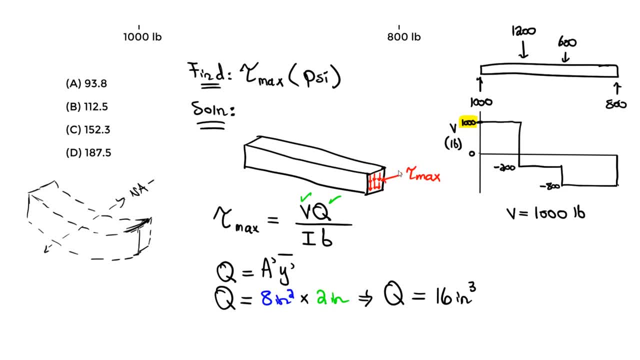 This is our neutral axis, which is going to be the X axis, X axis. So we have bending about that neutral axis, the X axis, And we know you just use I X, C, right? I X, the one for I X. 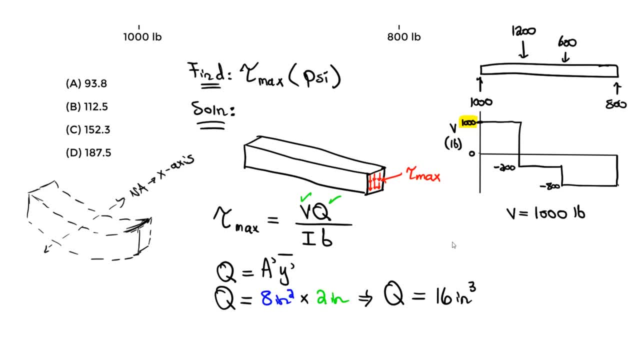 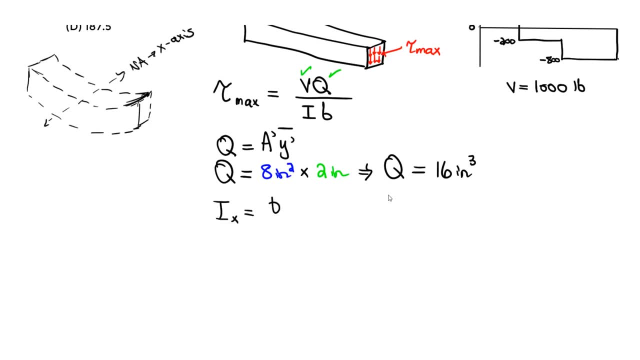 So for that one You look in the statics table. so you do. base times height to the third divided by 12.. Base times height to the third divided by 12, and that's going to be the I value. So base times height to the third divided by 12.. 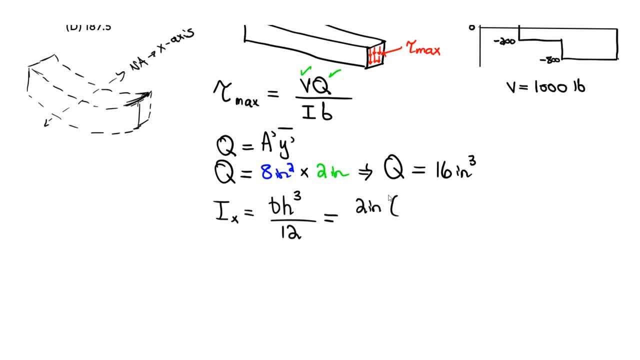 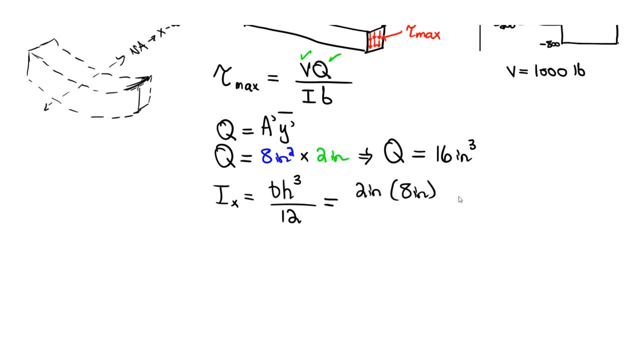 So the base you put two inches. The height is going to be what height? It's just the total height of the rectangle. So eight inches to the third divided by 12.. So now, doing the math for that, you should get about 85.. 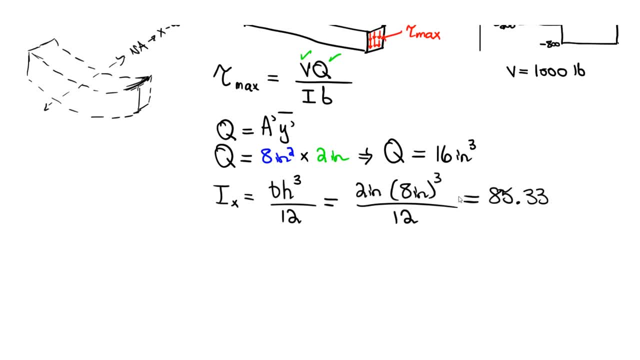 85.33 inches to the fourth. So that's going to be the first moment of inertia. sorry, the moment of inertia, the I value. Now for the B value. that's going to be quite simple, because B is just the width right. 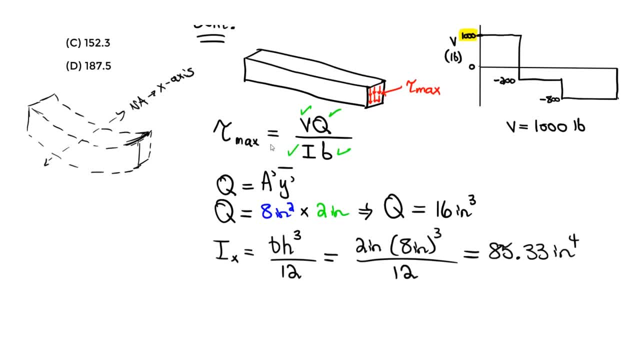 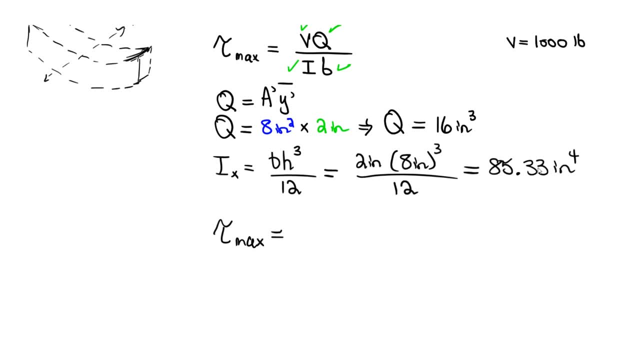 It's just two inches. two inches for B And we're done. So you just solve for tau max. So tau max equals to the B value. Again, what's the B value? Don't use the maxima. It's like external load. 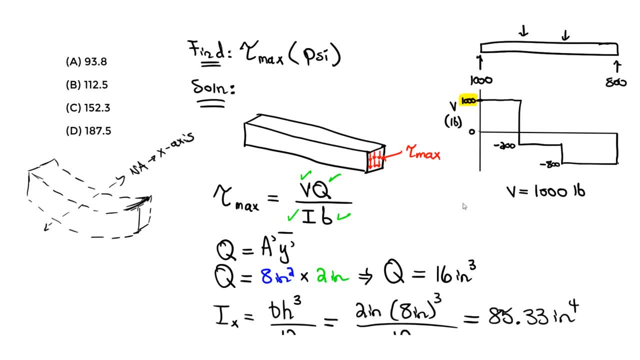 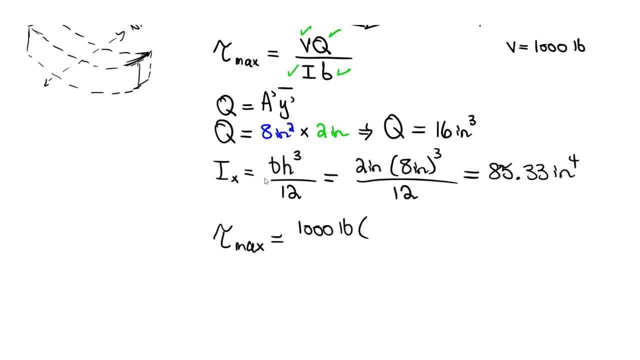 That's a typo and it's actually in there if you put that. but it's going to be the 1,000, right, Put that 1,000,. the maximum shear force: 1,000 pounds Q is going to be the 16 inches to the third divided by the I value. 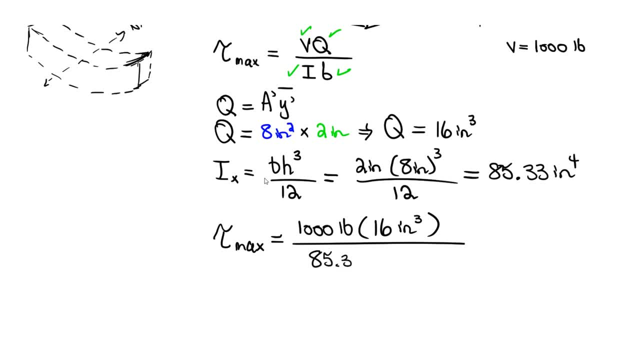 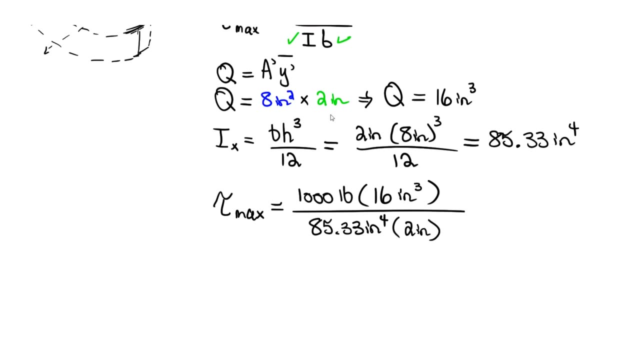 The I value is going to be this: 85.33 inches to the fourth. Then you multiply by the B value. The B value is how much? 85.33 inches to the fourth. The B value is going to be the width, and that's going to be two inches. 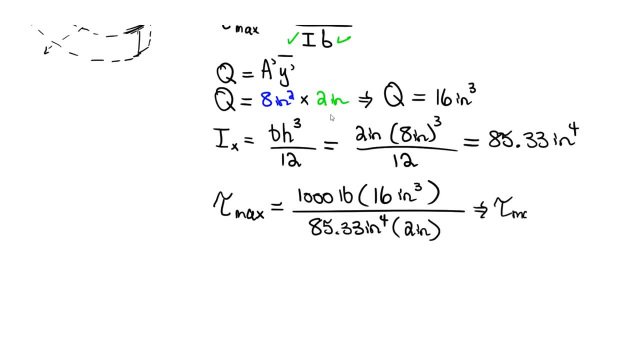 So now we solve for tau max. And if you do that, so let me do the math- You do 1,000 times 16 divided by 85.33, and you multiply by two And you get 93.75.. 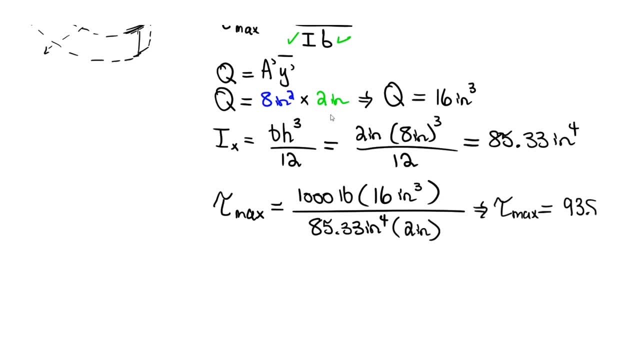 So it's about 93.8.. Okay, Okay, And you should get psi. right, You get psi, because the inches to the third here over inches to the fourth, this actually cancels This. just has a 1, right. 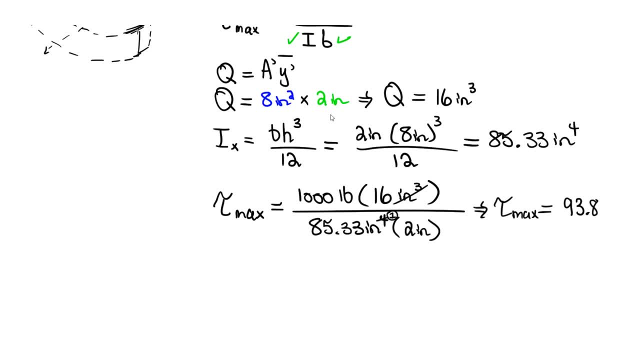 If you take the 3 over 4, you have that 1 left. So inches to the 1 is just the inch times. the inch is inch squared. You get pounds on tau. pound per inch squared is psi right. So that's going to be the answer for this one. 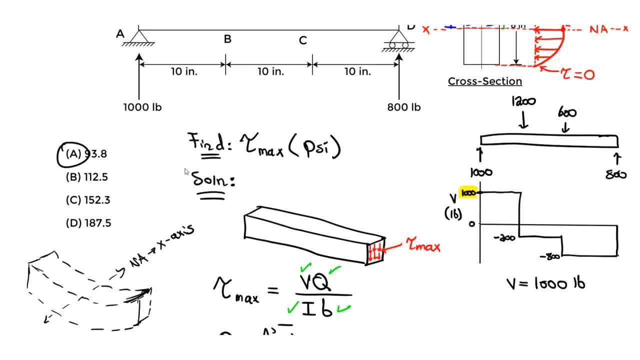 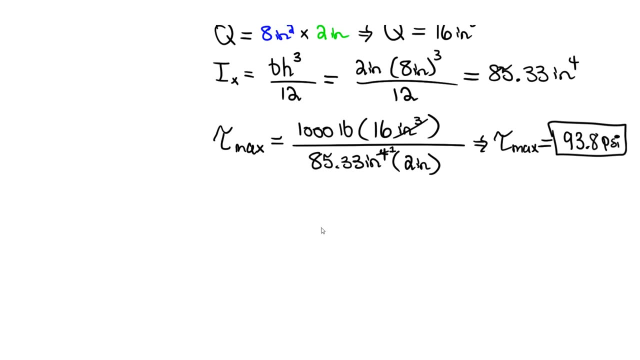 So 93.8 psi and that should be A for this. And I want to say real quick, some of you might have already known this, probably the mechanicals. You could have just actually used an equation that's not in the handbook to check your answer. 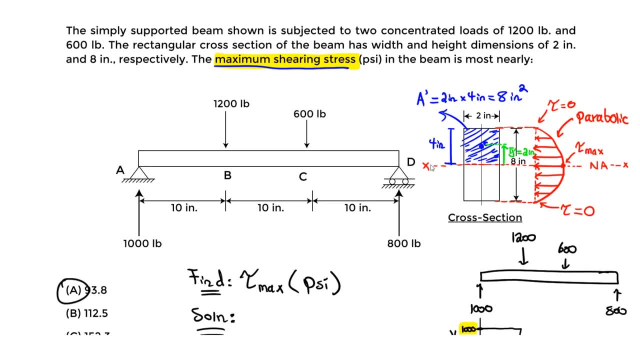 But obviously, okay, I want to say that you have to know, like the steps here, right, You have to know the procedure behind how you would do this, Just in case, like you get a T-shaped beam or an I-beam that's like non-symmetric or 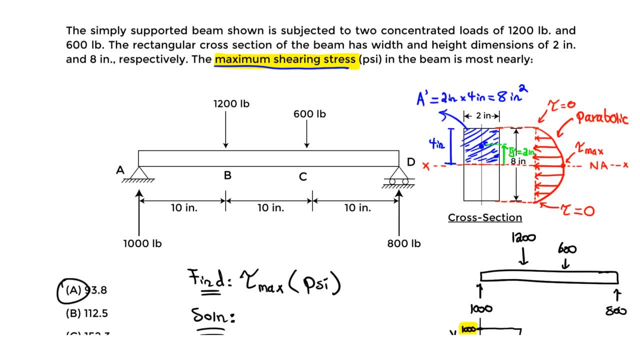 if you have a symmetric I-shape, there is an equation, but that's going to be. it's. the accuracy is like 15% off, So it's 15% lower than what you would get if you actually did the calculation. 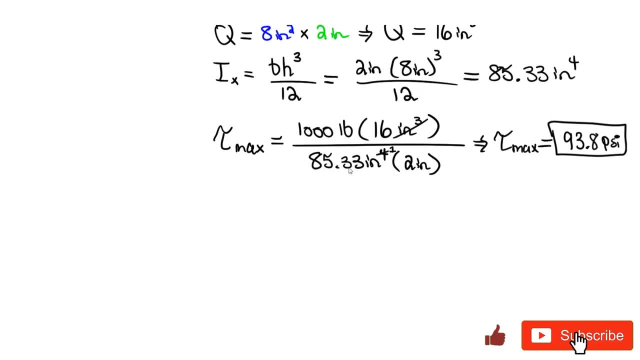 But here, if you just use this equation, you would get the same answer. So this is for a rectangle, Any rectangle. You can just use this equation. You take 3V divided by 2A, And A is just the area of the crossing, the total area. 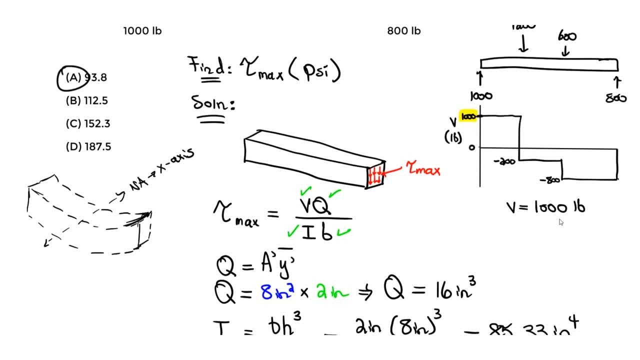 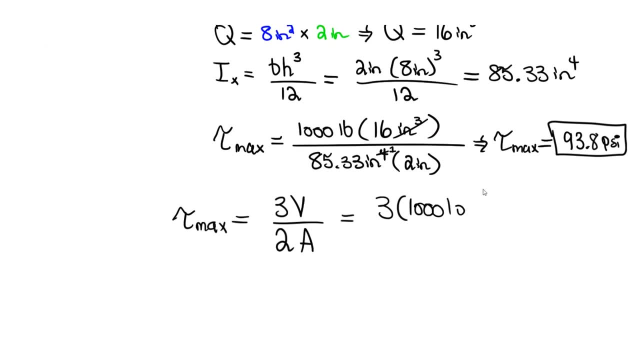 So let's do that. You take 3, what's V? V is still the value. we got right, That 1,000. So you would still have to do that step. So that's going to be 1,000 pounds. the maximum shear force: 2, what's the area? 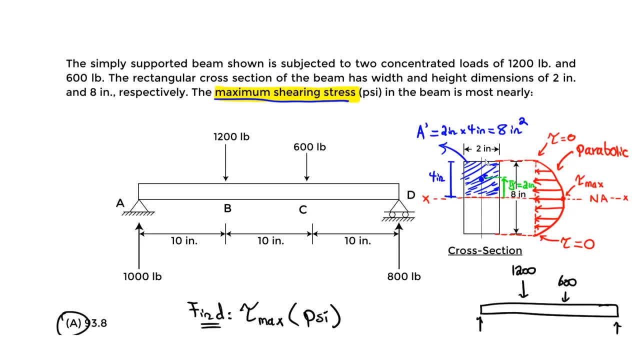 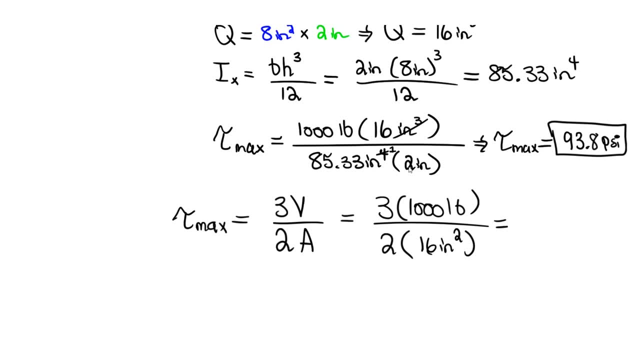 The area is simply, in this case, the 8 times 2.. So it's 16 inches squared, The area of the whole section. And if I do that, let me check, we should get the same answer. It should be exact, because this one's actually exact. 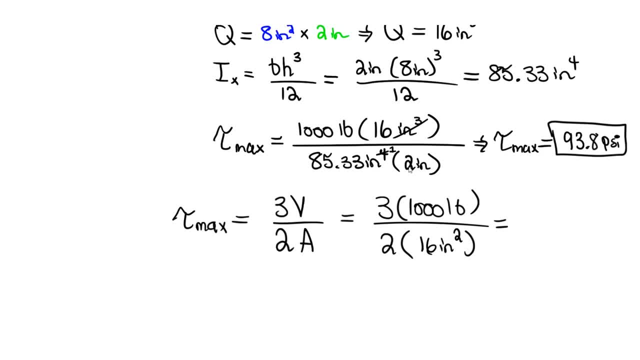 And when I do that I get 93.75.. So it's, yeah, 93.8, 93.75 psi. So this like this would save you a lot of time if you do indeed have a simple section like this one. 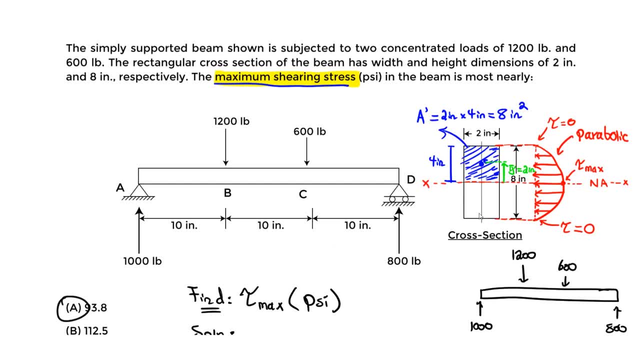 But this one's like to give you the foundational knowledge that you would, given you the exact steps of analysis, right, Just in case you do not get such a simple shape Like a rectangle, you might get a non-symmetric I-beam, a T-beam, whatever it may be. 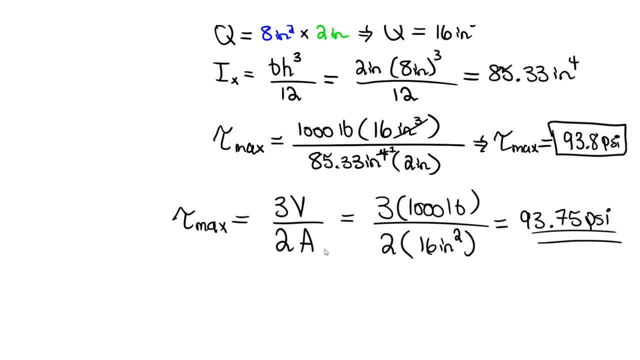 But you can indeed like just use this, right You want to. I would probably memorize this for the FE in case you get such a simple question, You can check your work, or you can actually just apply this and move on to the next section. 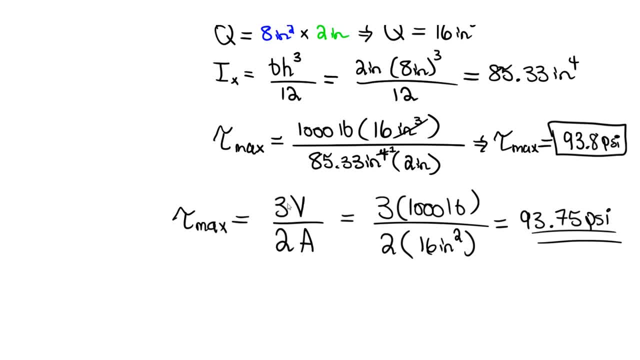